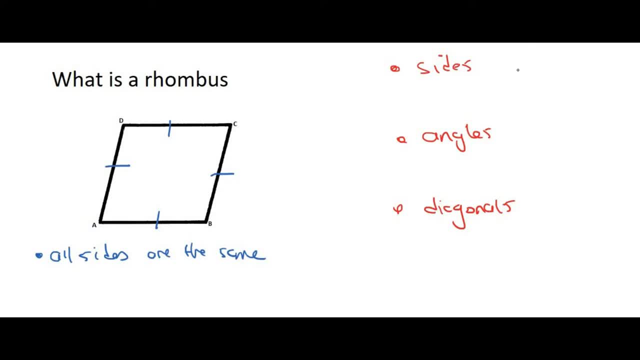 a nightmare. I mean, I just passed grade nine, Okay, so the sides are the same. Another thing we always have to look at with sides is: are they parallel? Well, yes, for a parallelogram they are parallel. I mean, for a rhombus they are all parallel. Okay, there we go. So we can say here that all sides are. 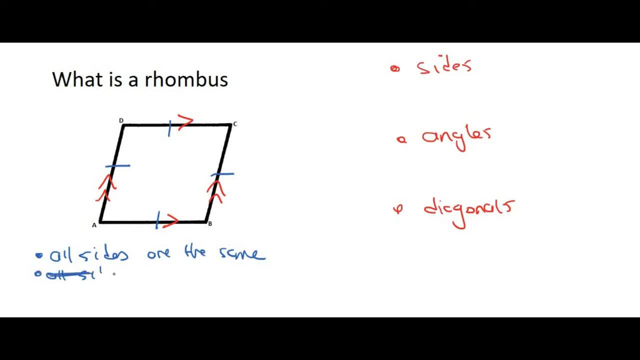 parallel Or no, not all sides. sorry, Two pairs of sides are parallel, Which means that these two are parallel And those two are parallel. They're not all parallel to each other. That can't happen. Okay, so we've looked at sides, Great Angles, Opposite angles. Let's take a look. Well, logically, 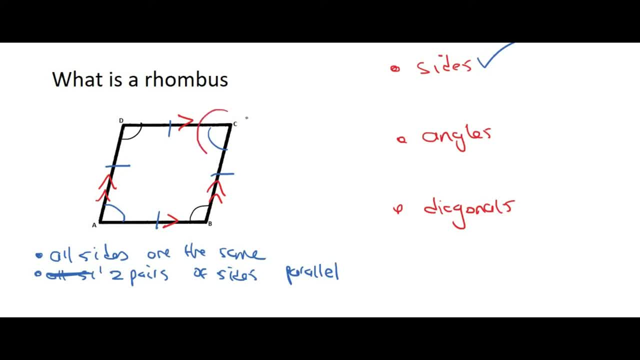 if you just have a look at this, If you look at this angle over here, you can see that it's less than 90 degrees, But if you look at this one here, you can see that it opens up more than 90 degrees. Okay, so we can't say that all the angles are the same, But what we definitely can say is that the 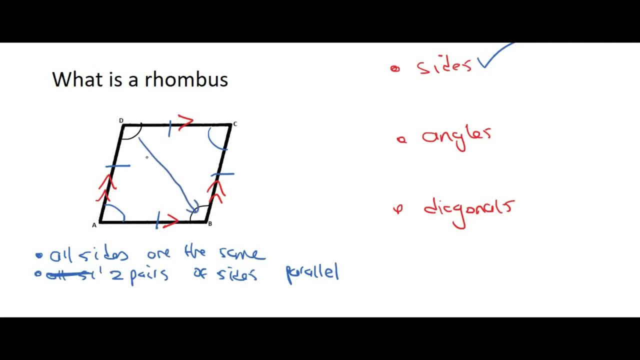 opposite angles are the same. Okay, so these are the opposite angles And these are the opposite angles, These two are the same- And then I'll show this with two little lines like that. And then those two are the same. Seriously, have a look at that, Like when you're sitting at home, Actually, look. 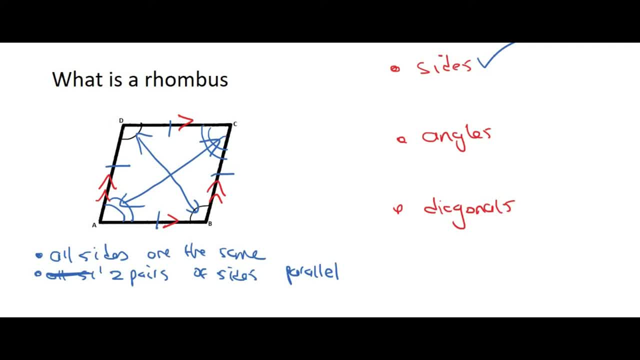 at it and you'll be like: oh right, it makes sense, The angles are not the same. Okay, so we've looked at the angles And so what we can say for that is two. Oh no, Opposite. Opposite angles are equal. 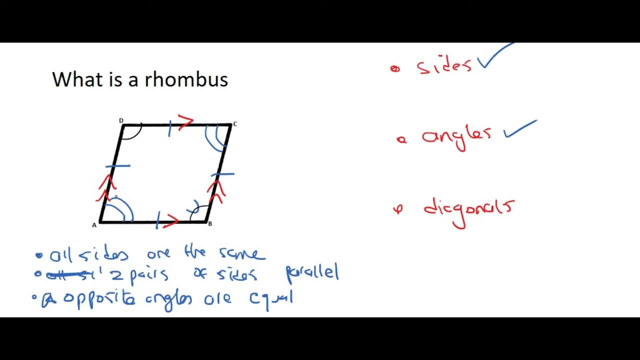 Okay, now we just need to look at the diagonals. So, with the diagonals, We'll just quickly draw them in. There we go, There we go. Now those diagonals are definitely not the same length. I mean, have a look at this. This one here is pretty long compared to this. 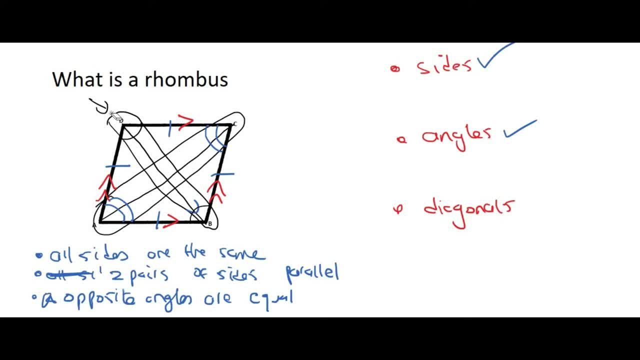 short little one going over there, right? So you must seriously just look at it. Don't memorize the stuff. Have a look at it, Like really stare at the picture and you'll realize. oh, it actually makes sense. So the diagonals are not the same. However, what we can see is that this half is going. 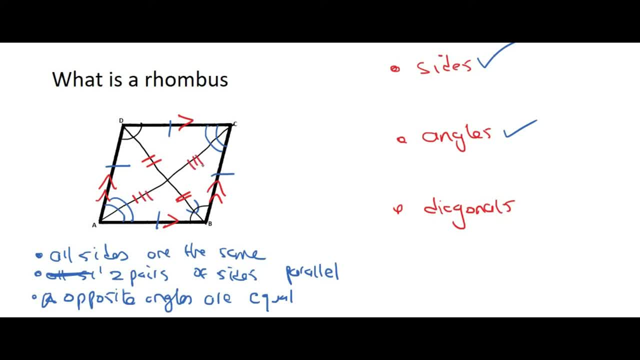 to be the same as this half, And this half is going to be the same as this half. So, Kevin, this pretty much looks like a parallelogram. I know It almost is a parallelogram. However, a parallelogram doesn't necessarily have 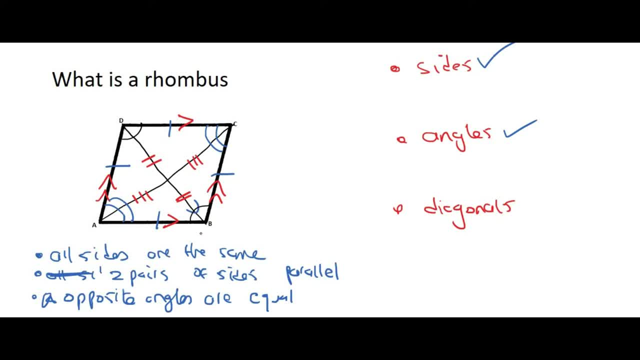 all four sides the same, But for a rhombus it has all four sides the same. That is the only difference. Now there's one little exception. Let's call it. Let's call it special features. Some special features about a rhombus is that these angles in the middle, they are all 90. 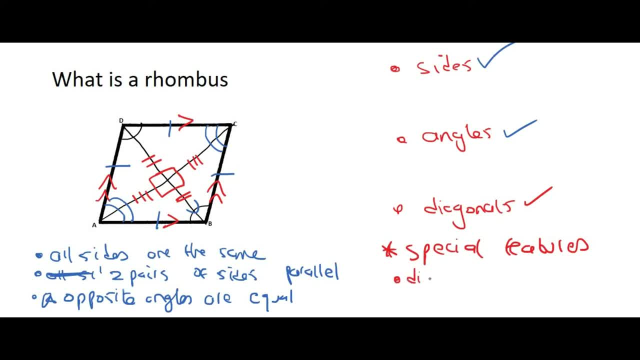 degrees. Okay, So we can say that diagonals bisect at 90 degrees. That's important. Should have added here in our little list of properties that the diagonals bisect each other, Meaning that the diagonals cut each other in half. Now, under the special properties, we can also say that the 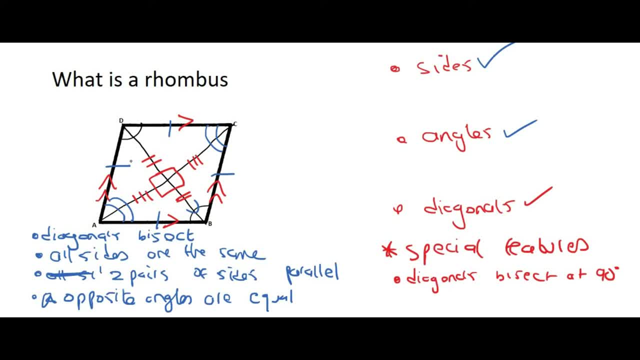 diagonals bisect at 90. That doesn't happen for a parallelogram. That's something special that a rhombus has. Something else that's really cool Is the corner angles are bisected. What that means is that these halves are the same. Okay, So that. 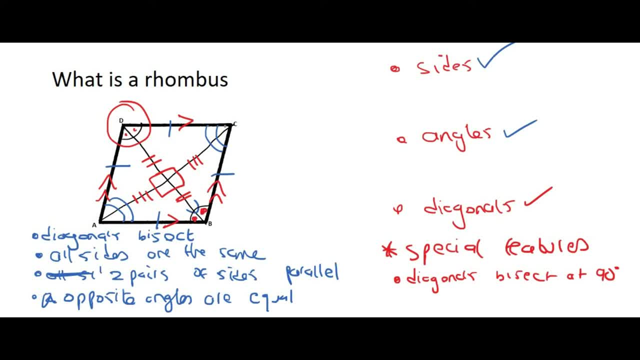 means these two halves will be the same down here, And then the corner angles up at the top and the bottom left. Their little pieces are also going to be the same, The little halves. Okay, So we can say that the corner angles are bisected, Corner angles are bisected. That isn't true for a 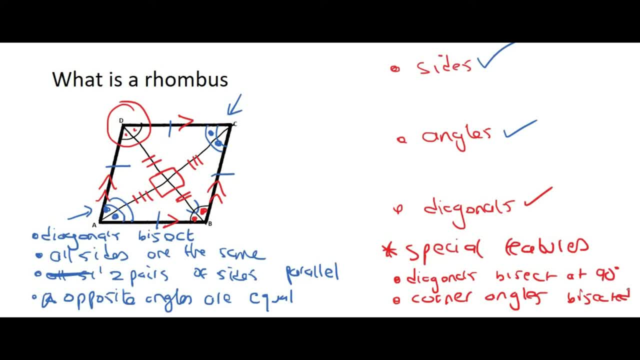 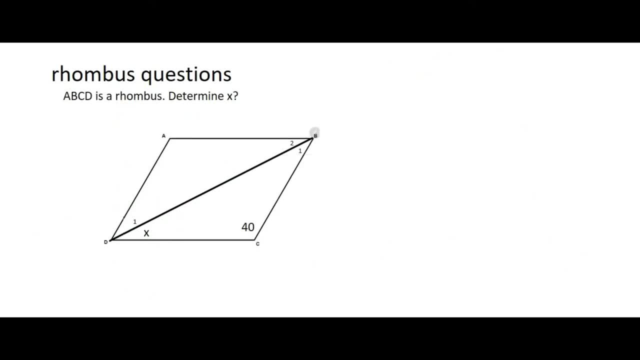 parallelogram, But for a rhombus it is. Okay, guys. So that's it for a rhombus. We're going to do some practice examples now, But these are the different properties that you need to know. So here's a rhombus question. They tell us that ABCD. 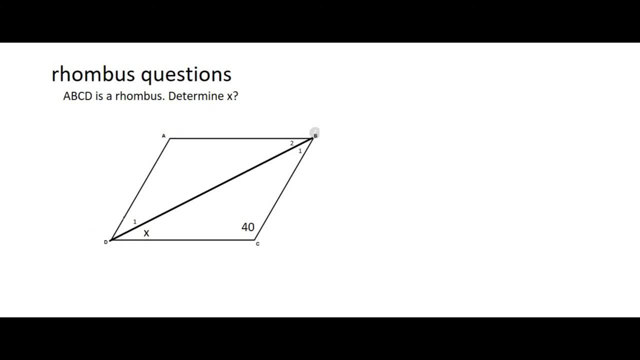 is a rhombus. Sorry for the small little letters. For some reason I couldn't get those to be any bigger. So if you need a magnifying glass, I would highly advise that. So it says here: determine the value of X, All right. Well, one way that we can do this is we could see that all the four sides. 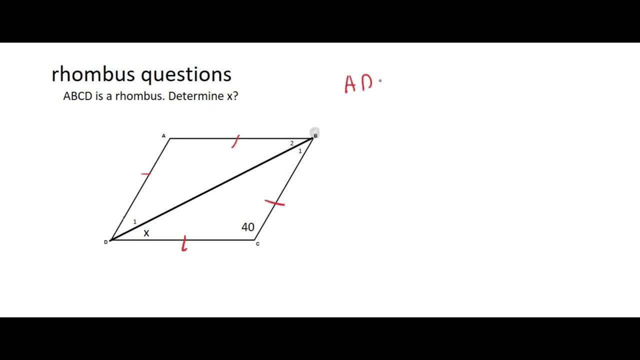 are going to be the same Right. So we can say that AD is going to be equal to AB, which is going to be equal to BC, which is going to be equal to DC. Why? Because these are the sides of rhombus, That's. 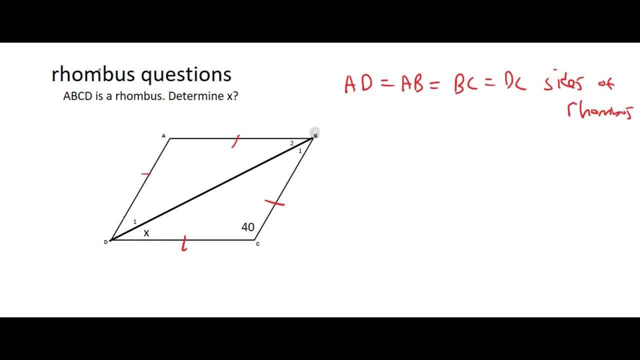 my reason, Sides of rhombus. We know that they are all the same. Now, why is this useful? Because this triangle over here is now isosceles, So we can now say that if you have an isosceles triangle, 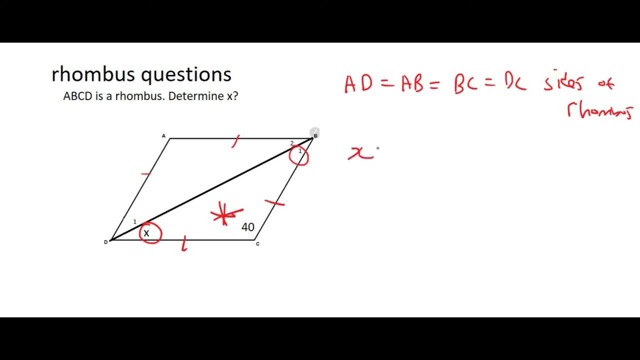 remember, the two angles will be the same, So we can say that X is equal to B1. And the reason for that is that the angles opposite equal sides. That's my reason. So I know that X is the same as B1.. 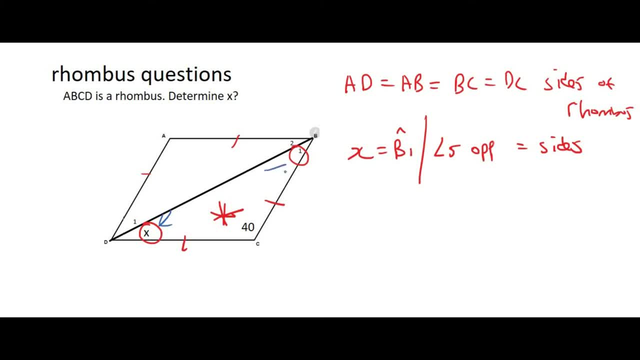 Okay, So does that make sense, guys? These, this angle and this angle, they are the same. So now it's very easy to find what X is, because I know that in a triangle all angles must add up to 180 degrees. This is already 40 degrees. So I could say that angle X plus angle B1 plus 40 should. 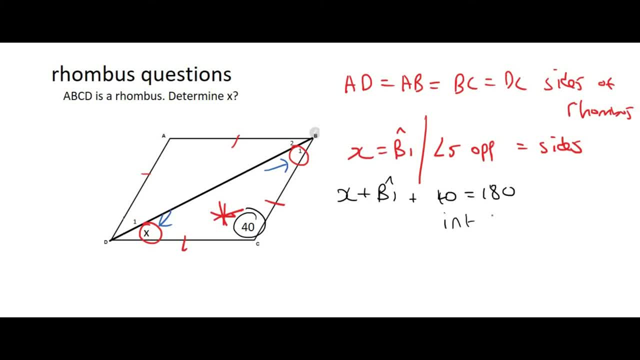 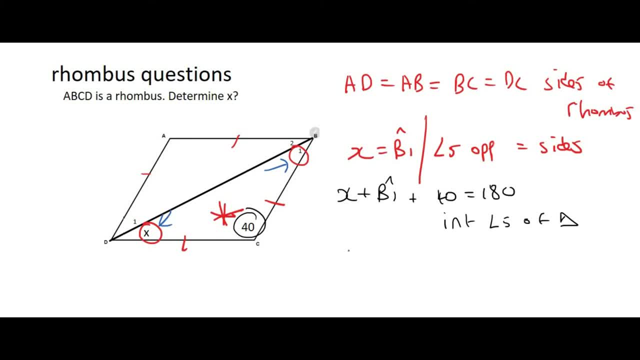 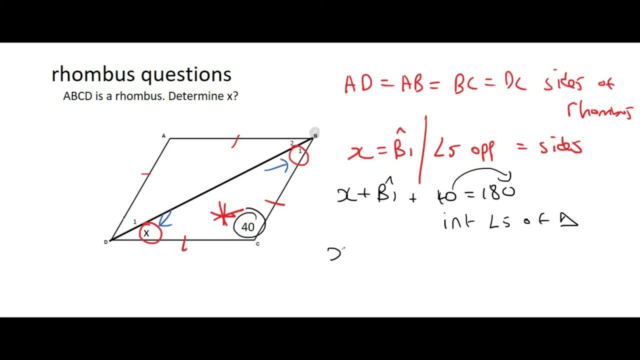 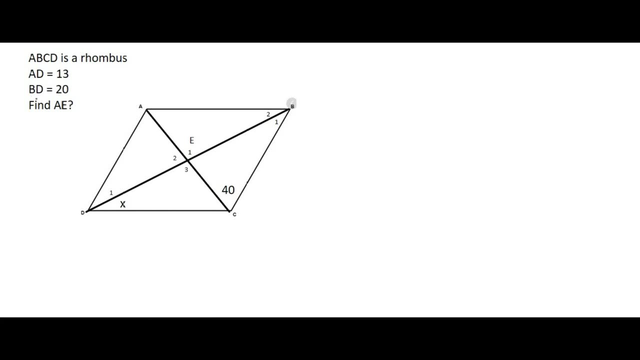 divide by 2, because they are the same, And so what we would find eventually is that angle X, or we can just say X, is equal to 70 degrees. Moving on to the next question, Here they tell us that ABCD is a rhombus. AD has a length of 13.. 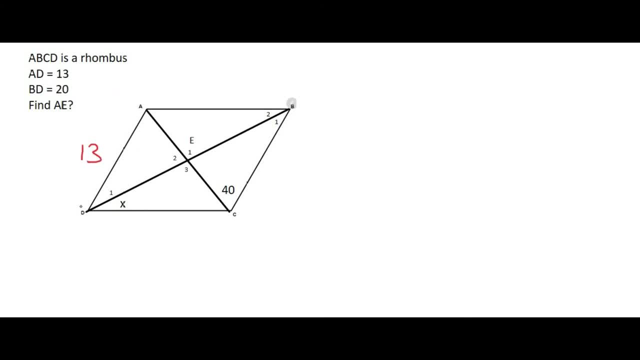 So I'm going to fill that in over here. BD. so this long diagonal over here has a length of 20.. Okay, so that entire diagonal is 20.. Find AE. So AE is this little guy over here? Or let me do it in. 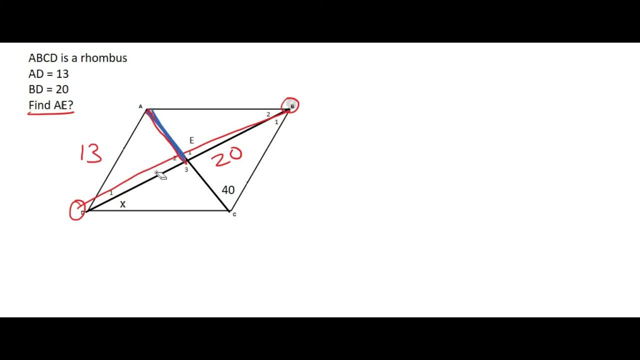 blue. So, AE, is that one over there? Now, here's the way to do a question like this. Whoops, I nearly raised the entire question. So what I want to show you guys is: have a look over here. If I do this and I do this. 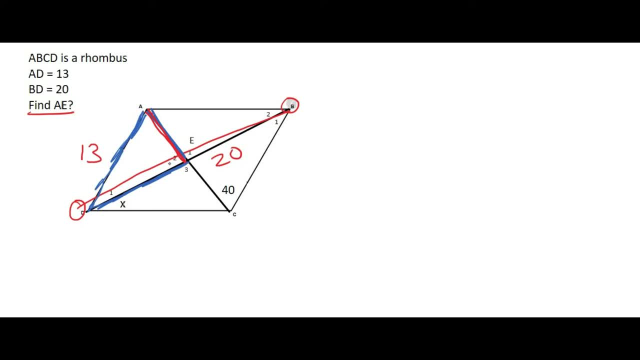 So what I want to do is I want to say that in the corner of the rhombus I have a 90 degree angle. Remember, we said that the special property of a rhombus is that it's corner angles are 90 degrees. 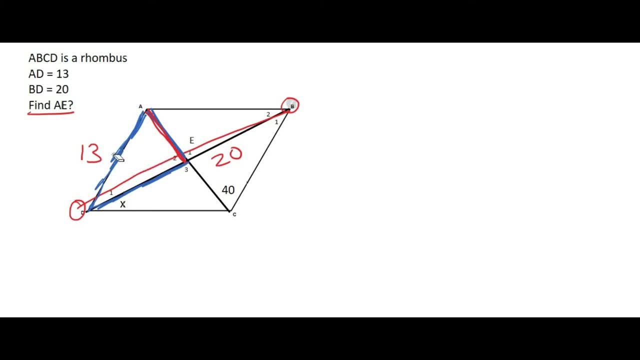 Aha, Okay, but I'm getting a little bit ahead of myself. But what we can do is we can say that angle E2 is 90 degrees. Why? Because that's just the special properties of the diagonals. So you say diags of rhombus. That's the reason you could use. Your teacher might use a slightly different.